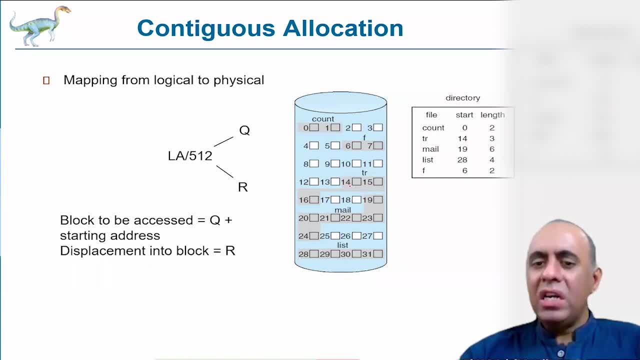 But there is a problem with this allocation that it does not allow to break the file into two groups of logical blocks, so that there is a problem that sometimes some small number of blocks get stuck inside two files. So these 17 and 18 you can see are stuck inside the file TR and mail and there can be only a file of size. two blocks can be stored on 17 and 18 and 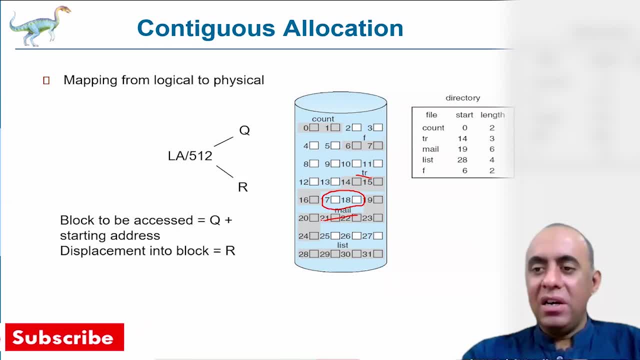 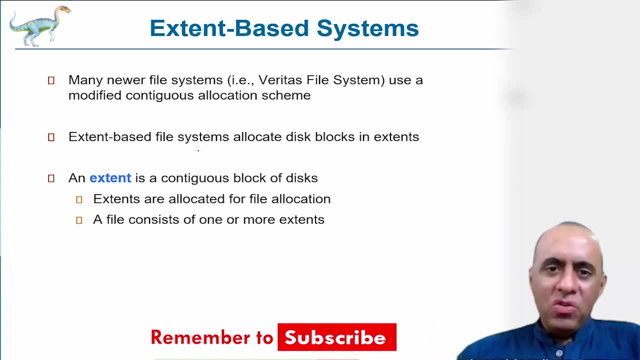 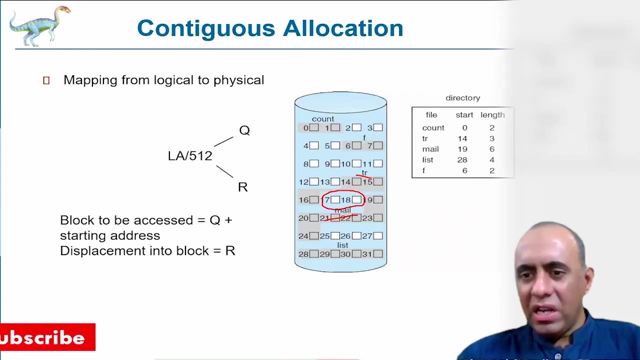 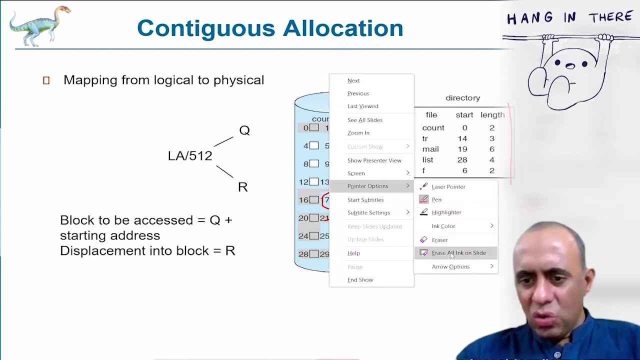 no bigger file can be stored on this in these two blocks. so, in order to get rid of this problem, what we do, we do. we can modify this into extent based system, where the directory structure will now contain more columns and more columns will now, uh, you know, store or save the information of. 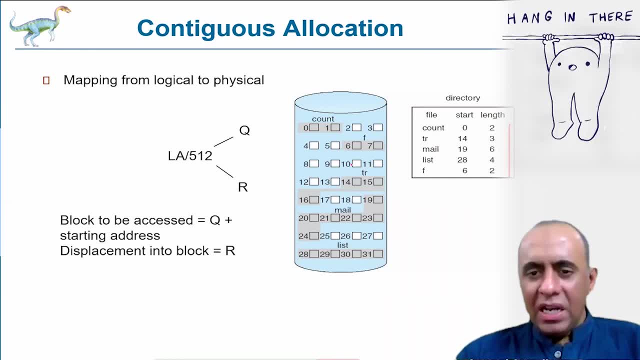 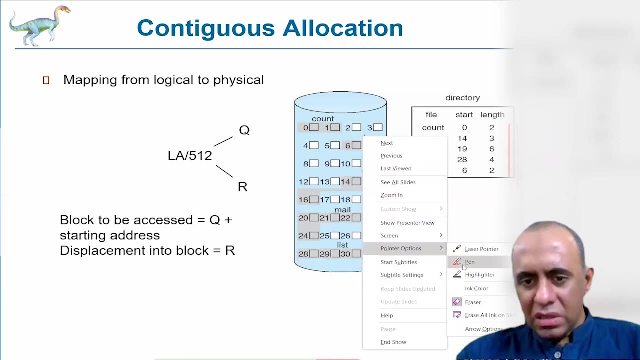 more extents. so now, for example, there was a file which i broke into two parts, and one part i stored over here and the other part, or maybe not here. let me erase this and let me use, uh, that the first file, the first part or first extent of the file i stored over here, and the second part or second. 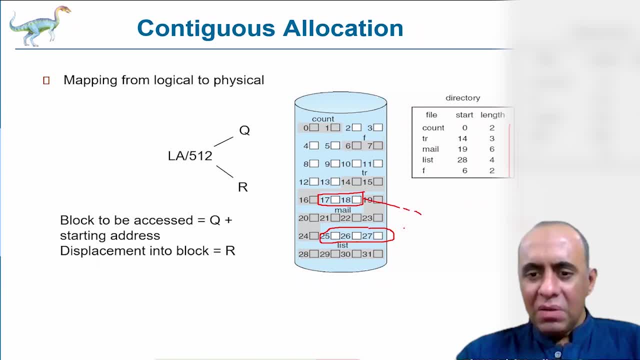 extent i stored over here. so both of these point to the same file. so, for example, the name of the file was a b. so in in front of a b, i will have to now write 17 and 2, and then i will be writing 25 and 3. so now, uh, this, uh, you know, file will be properly. 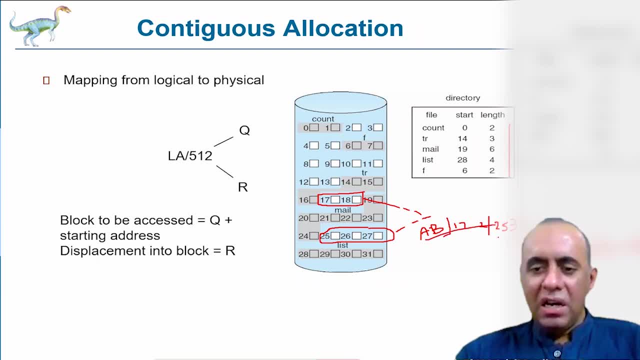 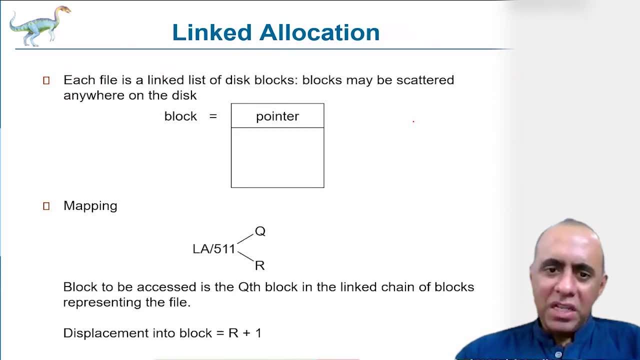 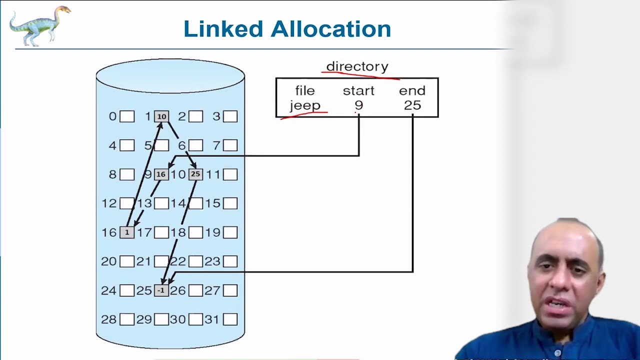 addressed by using the extent based uh scheme. so then there is another method, called linked method, in which you can see that the direct tightly contains the file name and in front of file name the uh starting block number and the ending block numbers are written, and it does. 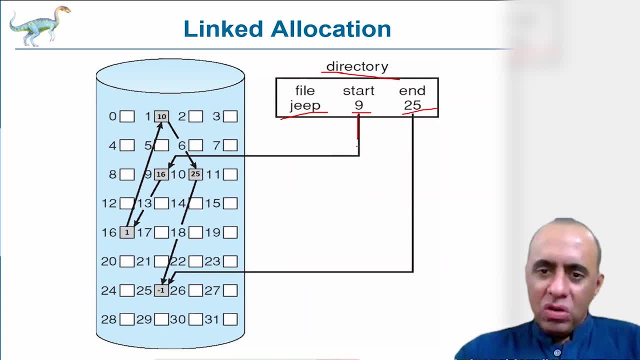 n't uh store the length of the file. so you go to the starting uh block, which is block number nine. inside the block number nine you also see the ending block number, which is block number 16.. so you go to block number sixteen, and in block number sixteen you see: 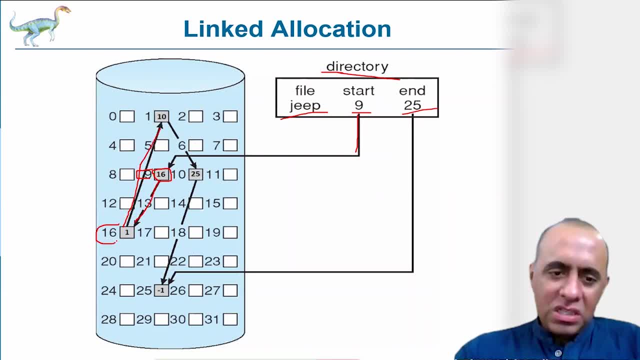 you're actually interacting as you%. block number seems as patterned and earnt and if we look at the here and there then both of them are same: undefined mean set ang extracting cell. you see the name of the next block in this file, which is block number one. so 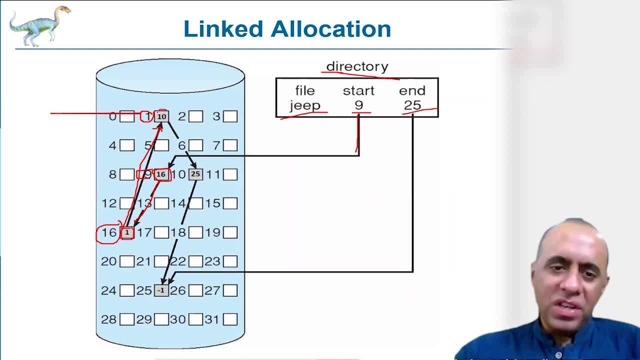 you go to block number one. inside block number one, you see the address or name of the next and, by the way, each block is now holding some data- most of the data of the file- and then a small one byte is may be used to store the next byte of. 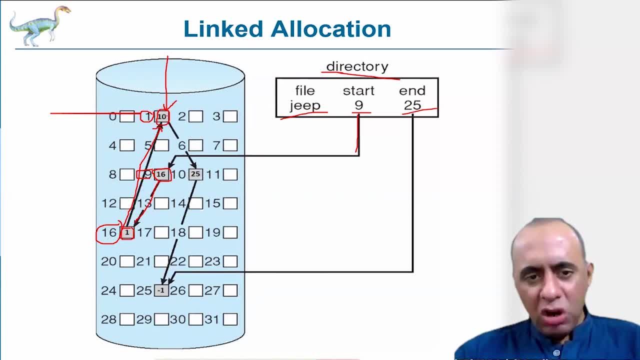 this you know file. so next, sorry, next block of this file. so next block is block number 10, you. so you go to block number 10, where there is file contents as well as name of the next block, which is block number 25. so you go to block. 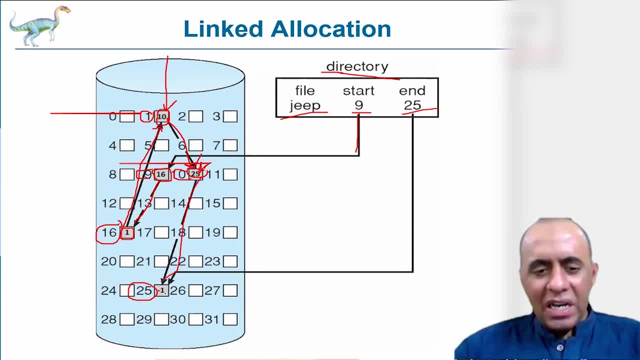 number 25. in block number 25 there is some file data and also there is minus one, and minus one indicates that it is not a valid block number, because block number starts from zero. so minus one means that this file has ended to this point and this end point also verifies that you have reached the end of the 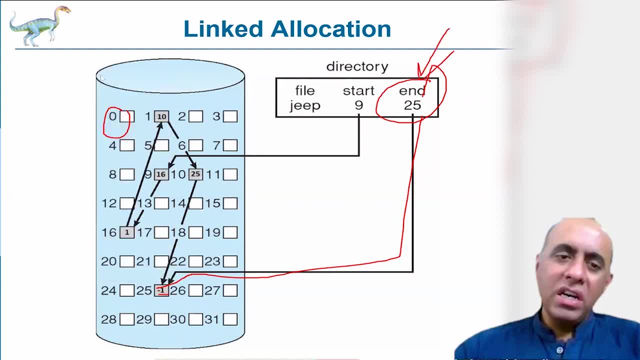 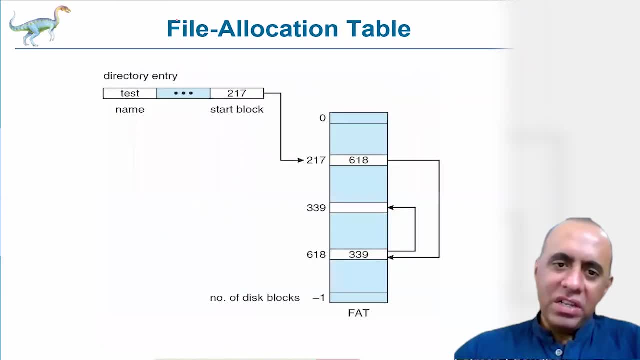 file. so this is the end point, and this is the end point and this is the end point file, although this information is redundant, but it also only gives you more reliability about the file. so this was called the linked allocation scheme and, by the way, your FAT or fad file system also used linked, you know. 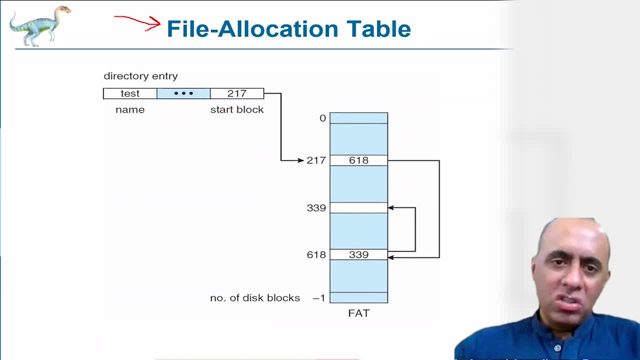 technique of allocation of logical blocks to the files, and here you can see the name of the directory and then you can see the starting block number only. it doesn't even store the ending block number. you go to that block number and this traversal is stored inside the fat array of all the block. 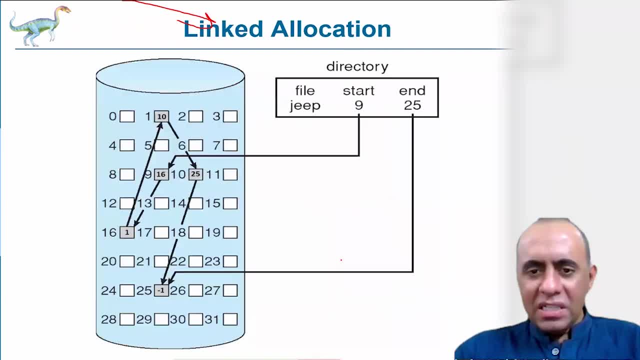 numbers and it gives you easier access. instead of storing these block numbers in actual data blocks, what have you done? you have created a copy of only block names over here and you are using the pointing inside this location. this is just a table of all of this blocks and it is easier to locate file numbers. 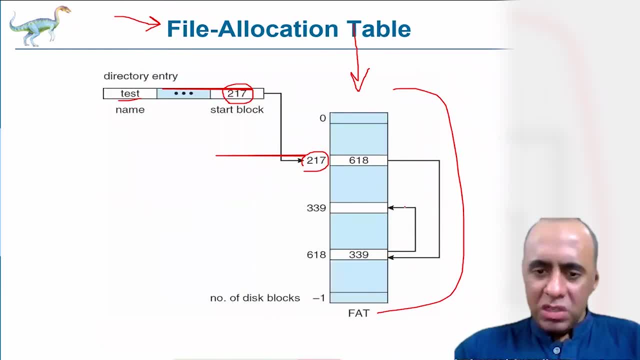 instead of going to the data blocks and then you can see that the data blocks are stored inside the data blocks and then reading the block number. so this is what fat did: slight modification of the linked scheme and you went to 217. 217 did not contain any data, but just the address of the next block, so you went to. 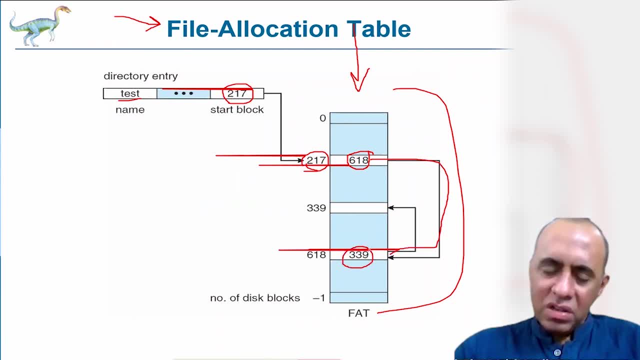 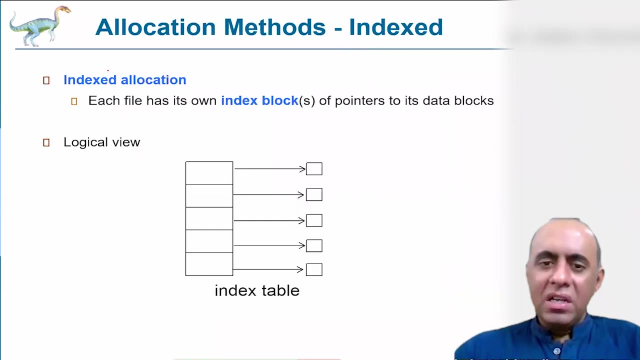 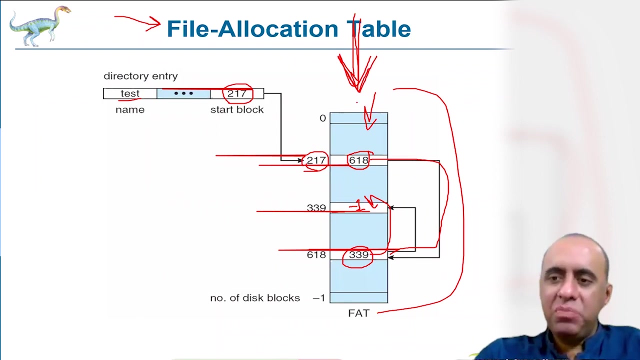 618. again, it is not the data, just the block number of pointer to the next block number, which is 339. so you are ending at 339. maybe you have to store minus 1 over here to tell this scheme that the file is ended by the way that this, this list of block numbers, contains the pointers and 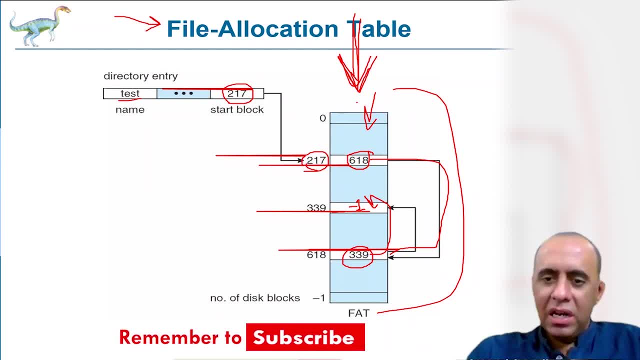 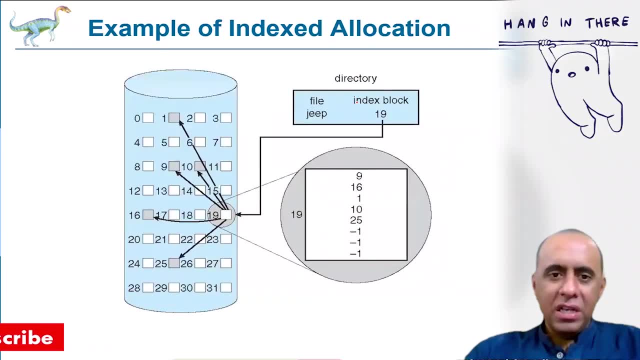 blocks for all the files, because because this list represents the complete hard disk just in terms of number numbers. so then there is another method called index location. the index location is even simpler because it simply contains the file name and the starting index box. so you can see here that the index is the two of the names of the block. 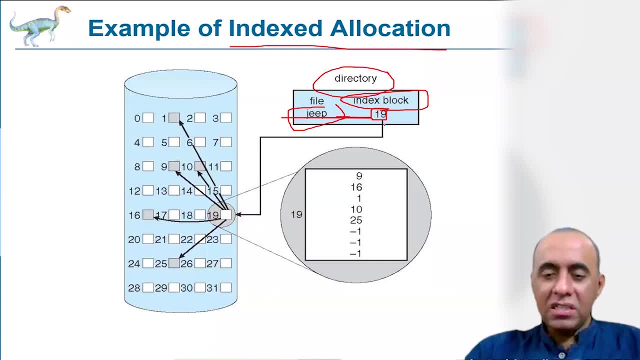 where the where, which is the index blocks, sorry, the name. that directory structure contains the name and the index block number and the index block is just another data block. if you zoom into that block you will see that it contains the actual, all the complete list of data blocks for this file, Jeep. so 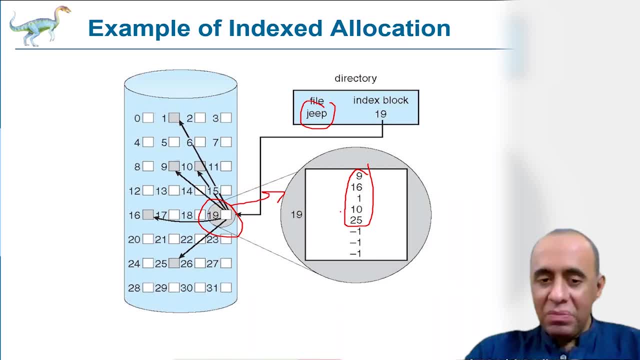 the benefit of it is it is that there will be no external fragmentation because every single block can be accessed, uh, individually, and the complete list is given in this data block and you simply, sorry, index block, and you simply save the name of this index block in the directory structure. 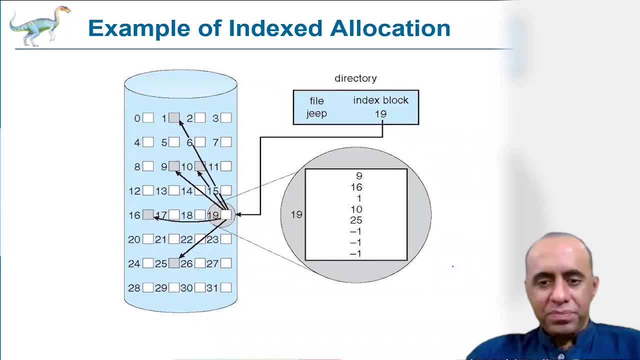 right. so this is quite convenient and, uh, because the the block numbers, sorry, the block size- is fixed length, just like we saw in, uh, in the memory, the paging technique in memory. for example, in this example the block height is eight. it is very important that all the 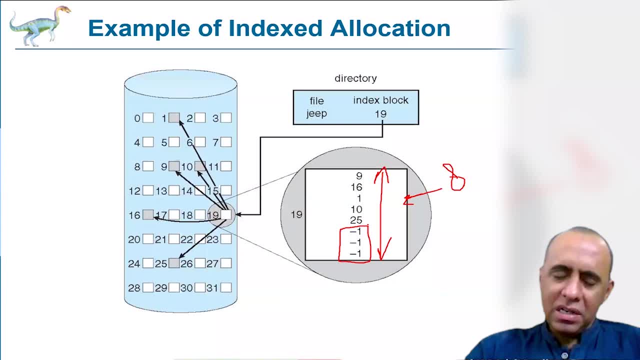 all the locations in this uh remaining locations which do not point to any uh. you know, blocks must be represented by minus one to tell the operating system that these are not pointing to any logical block size numbers. and we can, because these are data data lines, so you can actually store minus one over. 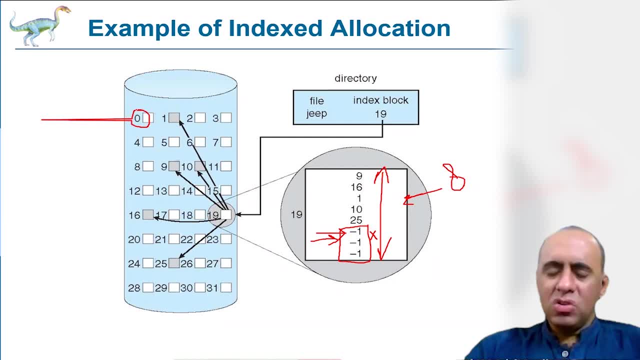 here and minus and block numbers start from zero. so minus one will not be pointing to any valid- uh, you know- block number. so, uh, you, you will readily know that this is the valid file index blocks. so my question to you: what would you, what would, what do you think we should do when? 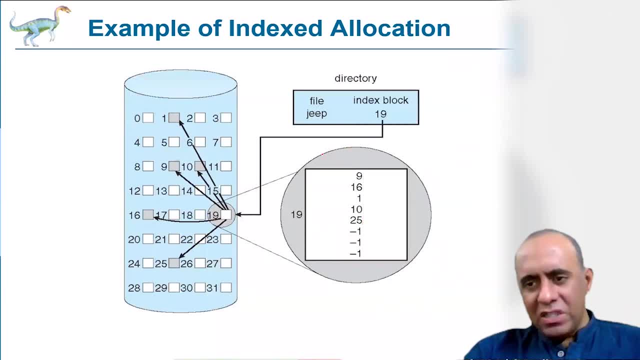 or if i want to make a file which is very large, which is 16 blocks wide or it it needs to have 16 blocks in it. so the answer to that would be that i can index only eight blocks using this one index block, but my file now needs 16 blocks, so i will need 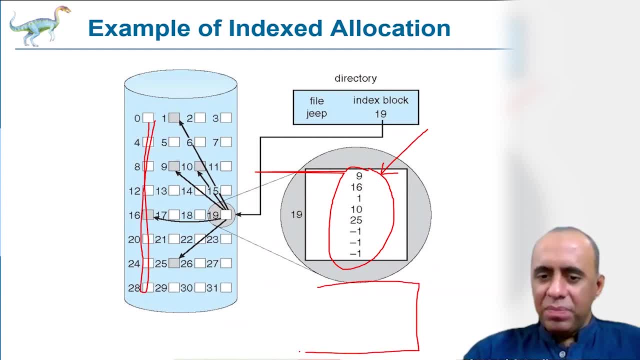 another index block right in which i will write the names of the remaining eight blocks. okay, so now the directory structure needs to do is: uh, do either of these two things either. it could store the name of the second index block as well. for example, the name of this block was 31, so it would store 31 over here. this was first option. 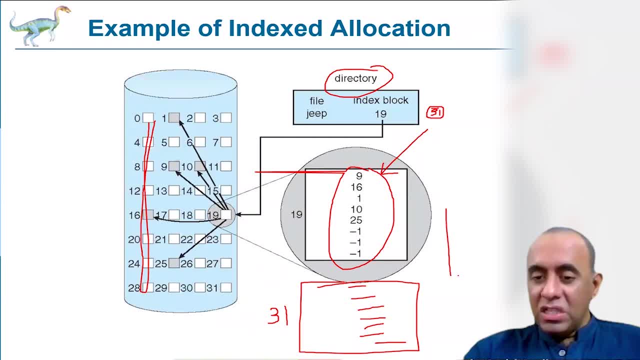 the second option could be that we use another data block as an index block and that outer layer index block points to these two index blocks, and then minus one in the rest of the entries, because this only contains two index blocks, and then the name of, for example, the name of this was 29. 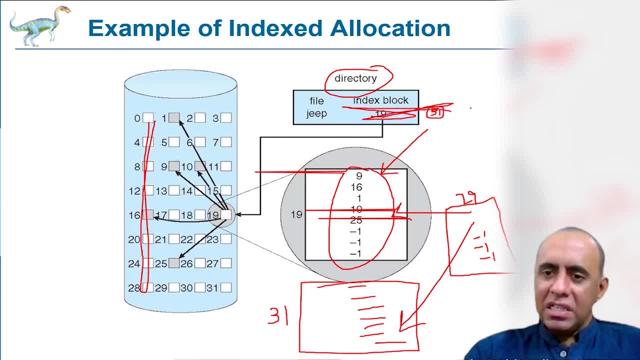 then all of this would be erased and then this 29 would be written in front of this directory and we would know that this is a two level directory scheme, so that it first reads the first block as not the direct access to logical blocks but access to the second level index blocks.